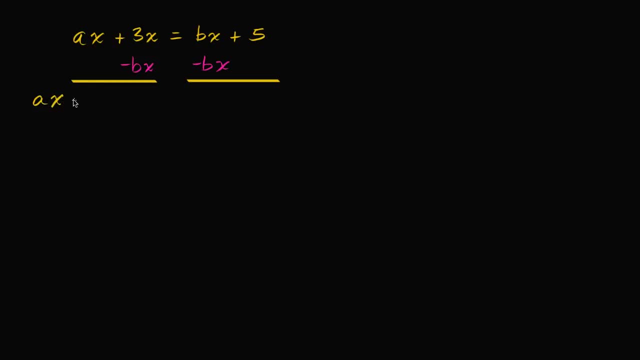 I'm going to have a on the left-hand side on ax plus 3x minus bx, So I can do that in that color for fun, Minus bx, And that's going to be equal to well: bx minus bx. 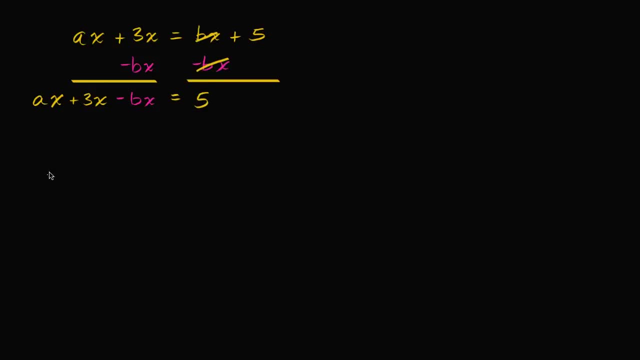 It's just 0, and I have 5.. It is equal to 5.. And now what I can do is I can factor an x out of this left-hand side of this equation, out of all of the terms, So I can rewrite this as x times well, ax divided by x is a. 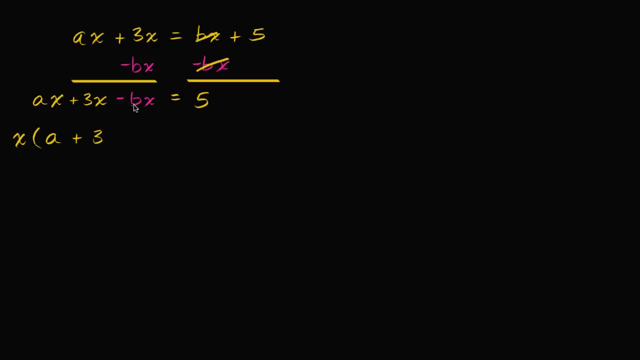 3x divided by x is 3.. And then negative bx divided by x is just going to be negative b. I can keep writing it in that pink color And that's all going to be equal to 5.. And now to solve for x, I can just divide both sides by. 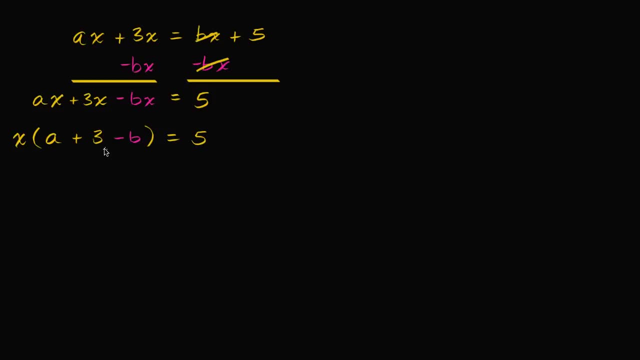 the thing that x is being multiplied by, by a plus 3 minus b, So I can divide both sides by a plus 3 minus b, a plus 3 minus b. On this side they cancel out And I have x is equal to 5 over a plus 3 minus b. 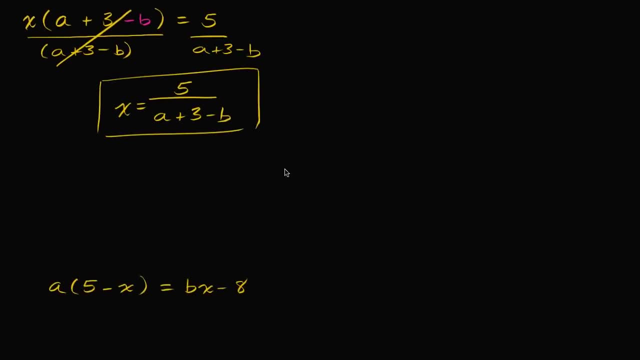 And I have a plus 3 minus b And we are done. Let's do one more of these. So another equation: Here we have a, here we have a times a quantity 5 minus x is equal to bx minus 8.. 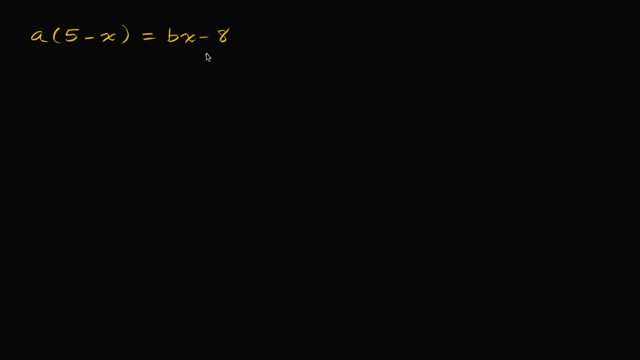 So, once again, pause the video and see if you can solve for x. Well, the way I like to approach these is: let's just expand everything all out. So let me just distribute this a and then I'm going to collect all the x terms on one side. 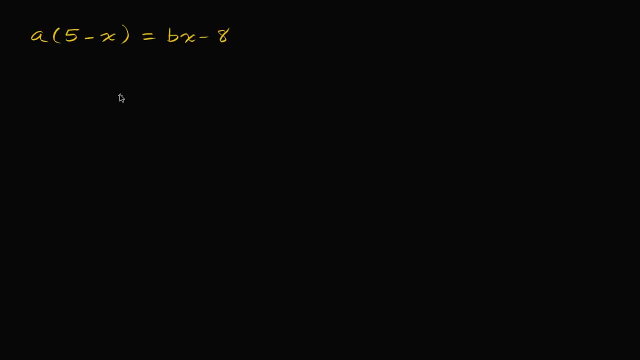 and all of the non-x terms on the other side and essentially do what I just did in the last example. So let's first distribute this a, So the left-hand side becomes 5a. I could say 8 times 5, or 5a minus ax. 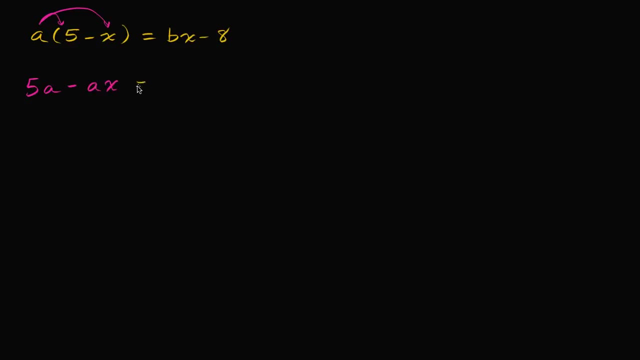 Ax, that is going to be equal to bx minus 8.. Now we can subtract bx from both sides. So we're going to subtract bx from the left-hand side, bx from the right-hand side And once again, the whole reason I'm doing that: I want all the x terms on the left and all the non-x terms on the right. 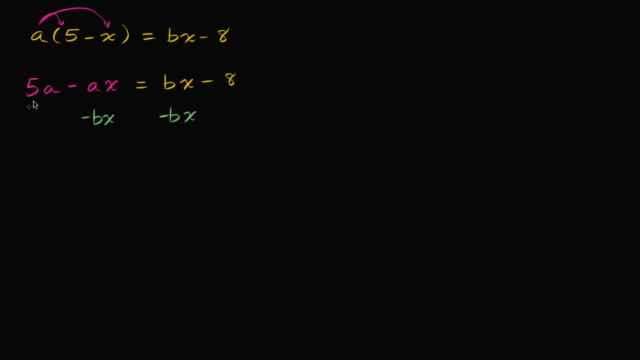 And actually, since I want all the non-x terms on the right, I can actually subtract 5a from both sides as well. So I'm kind of doing two steps at once here, but hopefully it makes sense. I'm trying to get rid of the bx here and I'm trying to get rid of the 5a here. 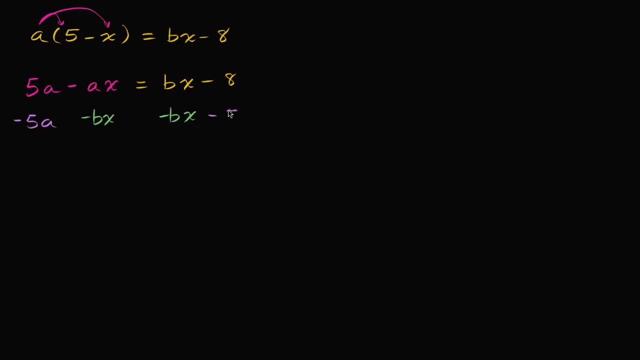 So I subtract 5a there and I'll subtract 5a there And then let's see what this gives us. So the 5a's cancel out, and on the left-hand side I have negative ax, negative ax minus bx. 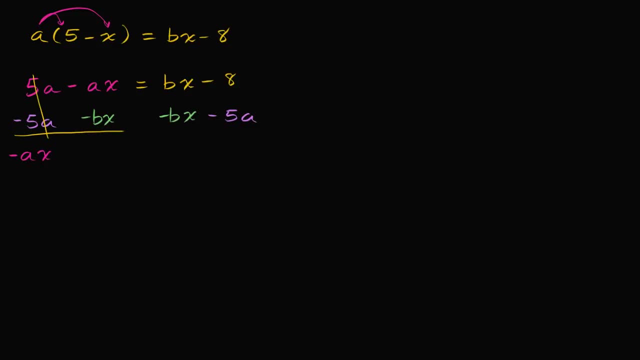 Minus. let me do that same green color minus bx. And on the right-hand side I have this is going to be equal to the bx's cancel out and I have negative 8 minus 5a. Negative 8 minus: let me do that. same magenta color minus 5a. 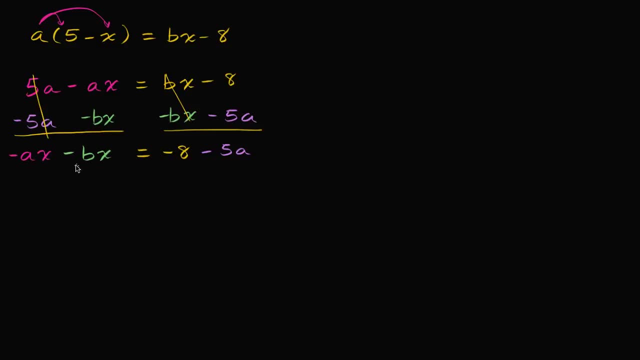 And let's see both I've now. I have all my x's on one side, all my non-x's on the other, And here I can factor out an x. And if I factor out an x, what do I have? 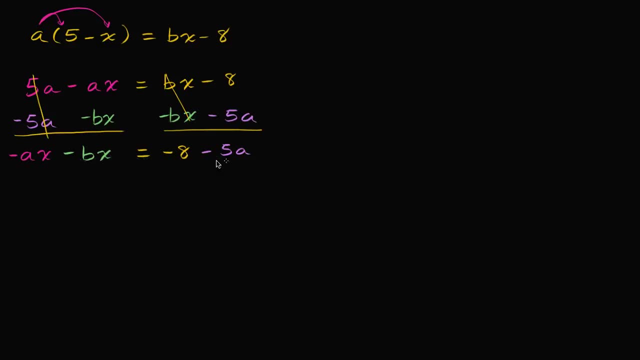 And actually one thing that might be nice: let me just multiply both sides by negative 1.. If I multiply both sides by negative 1, I get ax plus bx. plus bx is equal to 8 plus 5a. That just gets rid of all of those negative signs. 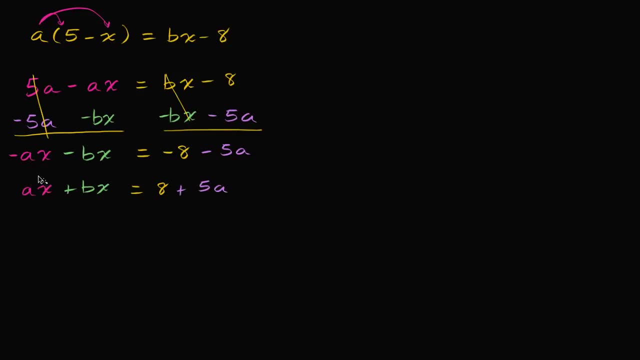 And now I can factor out an x here. So let me factor out an x And I get x times a plus b. a plus b is going to be equal to 8 plus 5a. 8 plus 5a and we're in the home stretch now. 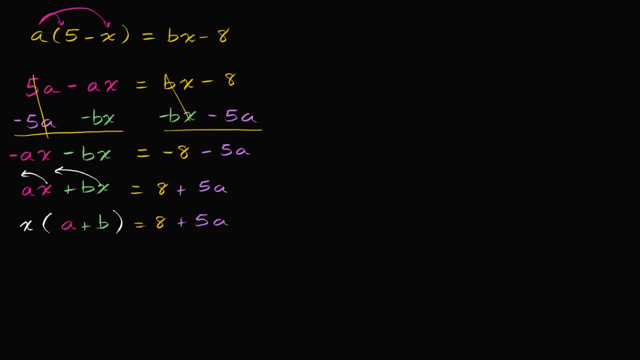 We can just divide both sides by a plus b. So we can divide both sides by a plus b And we're going to be left with: x is equal to 8 plus 5a plus 5a over over, and actually I'll write a and b in our original colors.